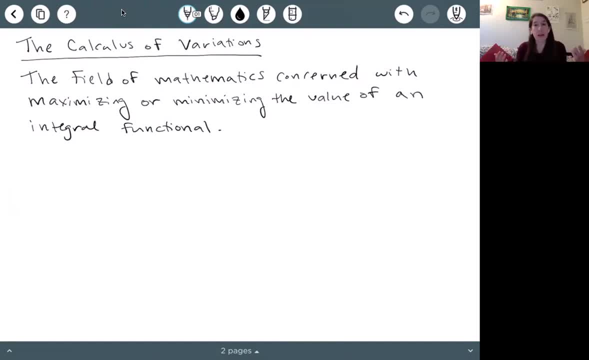 minimizing just a function, where you take the derivative of that function and set it equal to zero. But here we're trying to maximize or minimize the value of an integral functional, which is going to be slightly more complicated. And so what I'm talking about here is if we have 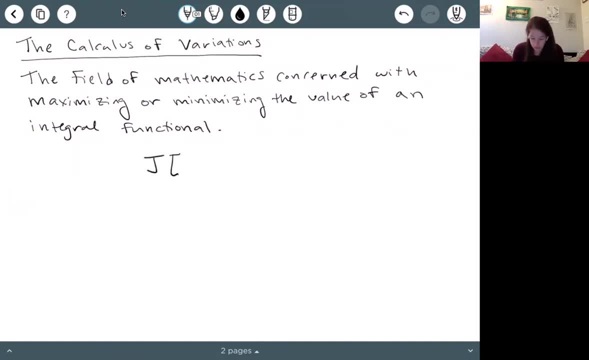 some functional j, which is a function of the function x of t, where it's an integral functional. So we're integrating from some time, for instance t a to t b, and although it doesn't have to be time, it could be some other type of. 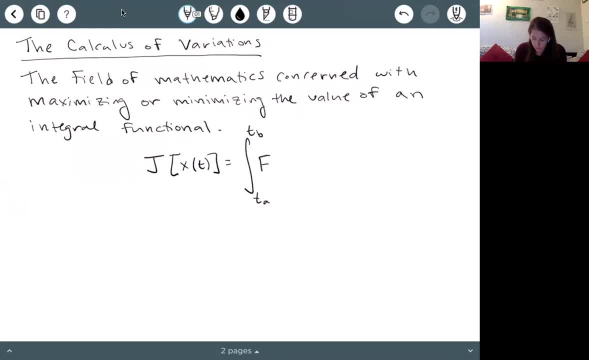 variable of some function, where this is a function of potentially x, of t, the derivative, the time derivative of x, and then also t itself, and then where we're integrating over time here. So we're trying to figure out the function. 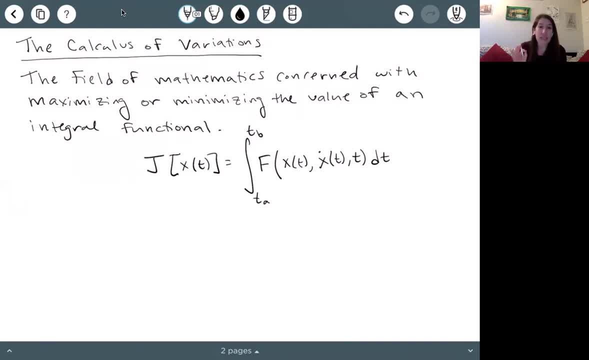 x of t. we're trying to find the function x of t that extremizes the integral of f, where here f is some function of x, x, dot and t. We're trying to find the value or the function x that extremizes j. All right, so this is a fairly complicated problem that we're trying to answer. 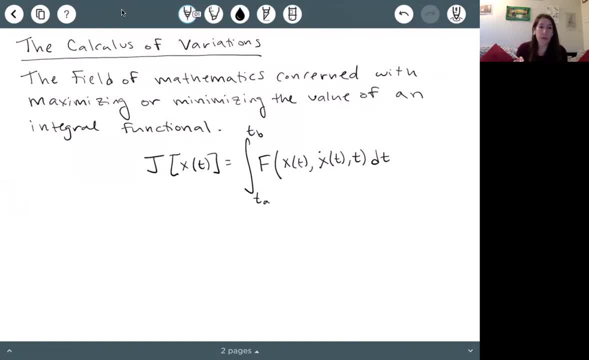 here, And I'm not going to prove for you what the answer, how to do this, but I'll show you what's known as the Euler-Lagrange equation, which is a solution to this problem of how to find the function x of t which extremizes j. 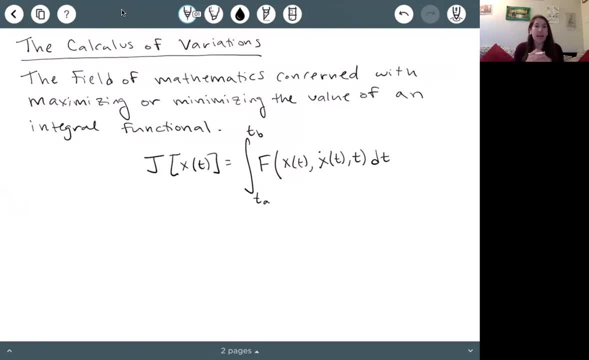 But before I do that, I just wanted to sort of give you an idea of where calculus of variations is important in physics, because you could just look at this as simply a math problem. You're trying to do this extremizing math, But it turns out to be quite commonplace in physics where it turns out that nature: 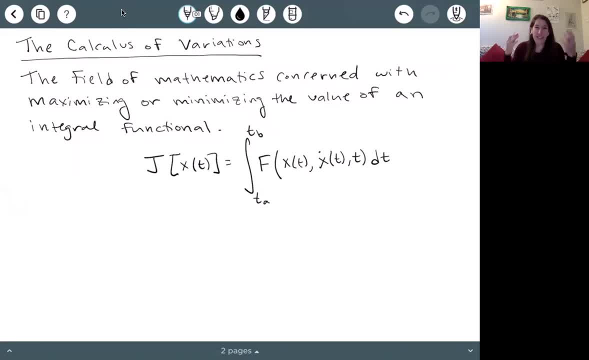 likes the extremum of things. so the solution to many physics problems is that you need to extremize some integral functional. So examples where it comes up. so maybe you've seen in optics Fermat's principle which tells us that light, the power of light, can be extremely important, but you need to 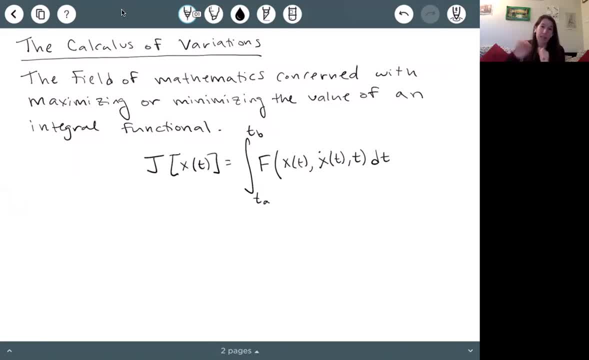 that a ray of light will take is the path of shortest time. Another place that it comes up is in general relativity. So the paths that particles follow in general relativity extremize what's known as the proper time along that path And then in classical mechanics. 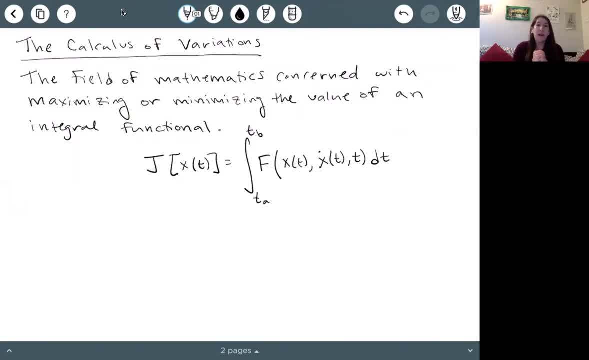 so for us it'll be important because in Lagrangian's formulation of classical mechanics it turns out that the trajectories of particles, or trajectories, really, of systems, are given by the extremum of what's known as the action of that system, and we'll see more about that in the future videos. 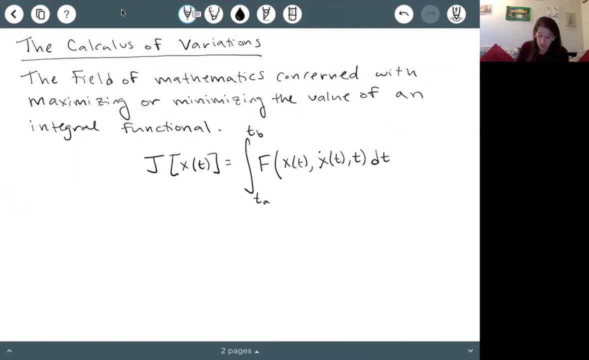 So the general solution to this is given by what's known as the Euler-Lagrange equation, And it's the Euler-Lagrange equation and it's the direct derivative of the partial derivative of the function f. So, if we take the time, derivative of the partial derivative of this. 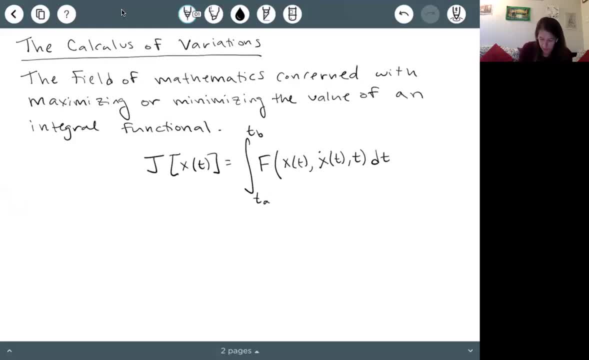 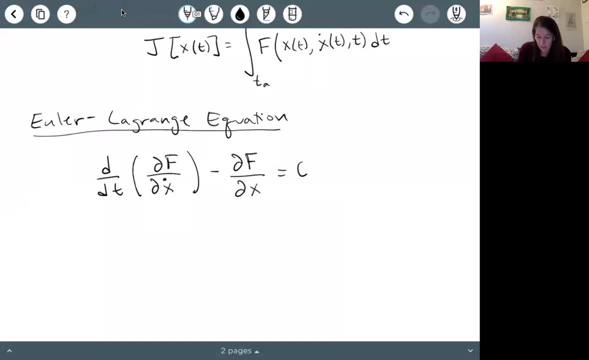 function f with respect to x, dot and then subtract the partial derivative of f with respect to x, and then this is a differential equation, ultimately, that we can solve for x, then that function x, subject to whatever boundary conditions we might have, will be an extremum of j, or a will be the extremum. 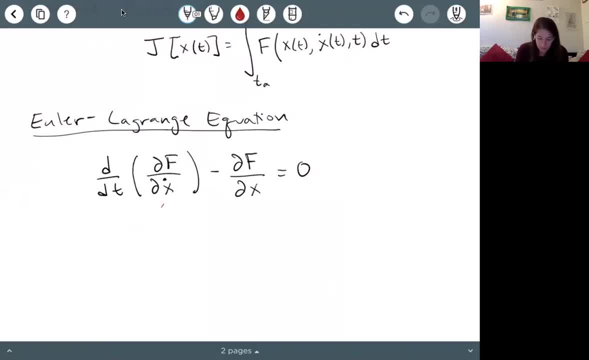 So something very important that I want to point out here is: in these partial derivatives you're going to treat x and x-dot as though they are independent variables, which might sound strange. but so when you take the partial derivative and you're going to treat x as an independent variable, 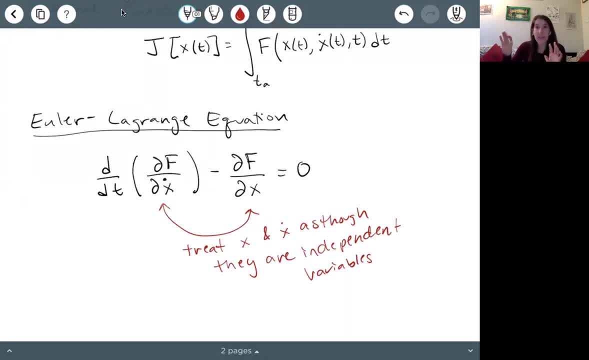 and you're going to treat x as an independent variable. you hold everything fixed. In this first guy, you hold x fixed and take the derivative with respect to x-dot. and then, in the second term, you hold x-dot fixed and take the derivative with respect to x. 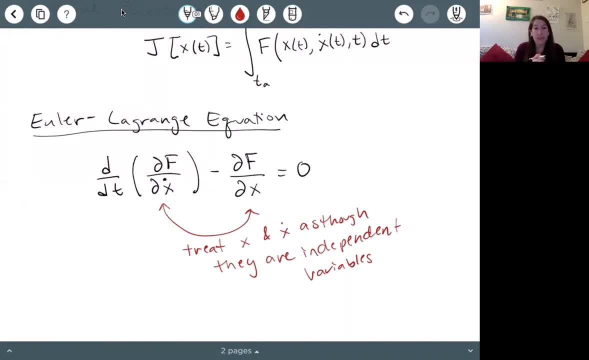 so you're treating x and x-dot as though they are independent variables of our function f, And then the solution to this again will extremize the function j. So the last thing I want to do is is just give you an example of the types of problems. 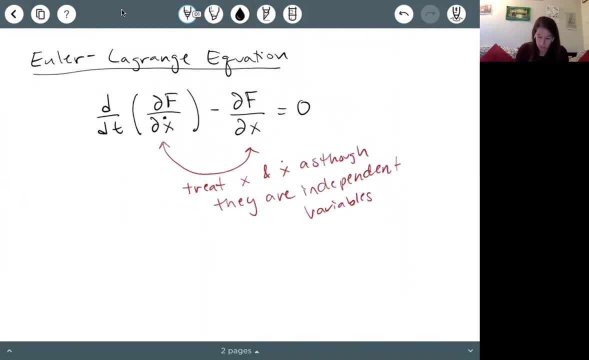 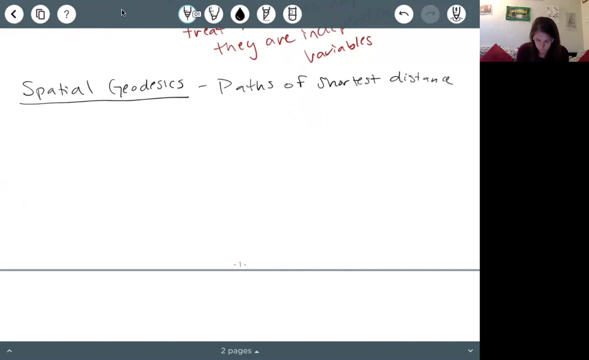 that we use the Euler-Lagrange equation for. And specifically, I'll give you an example of geodesics in space. So these are spatial geodesics, which are simply the paths of shortest distance between two points, So, for instance, in flat space. 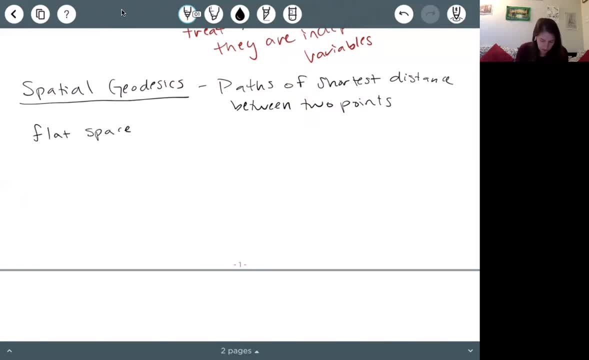 if we have some point A and B and we want to find the path of shortest distance between two points, we're going to use the Euler-Lagrange equation for that. So we're going to use the Euler-Lagrange equation for that. 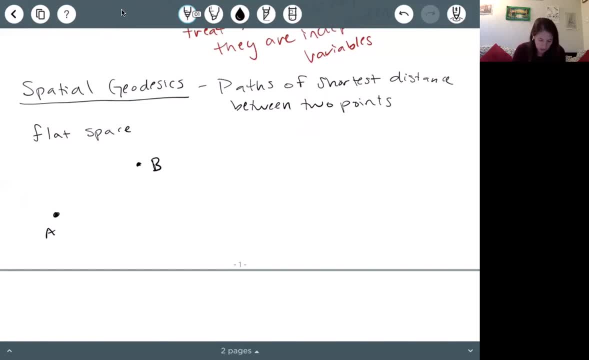 Probably most of us already know the answer to this question, which is that it's just going to be a straight line. So this would be the geodesic And you can imagine if we took any slight variation from that short line, any type of variation we might want, right? 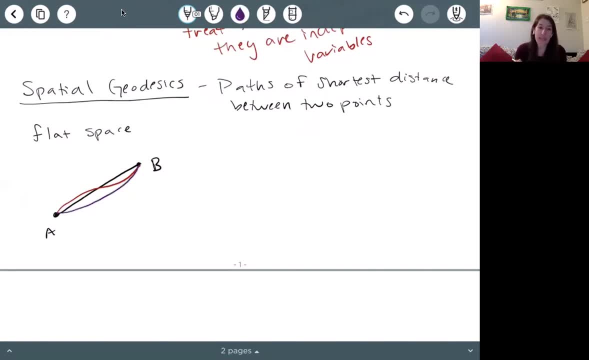 any of these paths are going to be longer than the straight line distance. So we would say this black line is the geodesic subject to the short line And this is the geodesic that starts at point A and ends at point B. 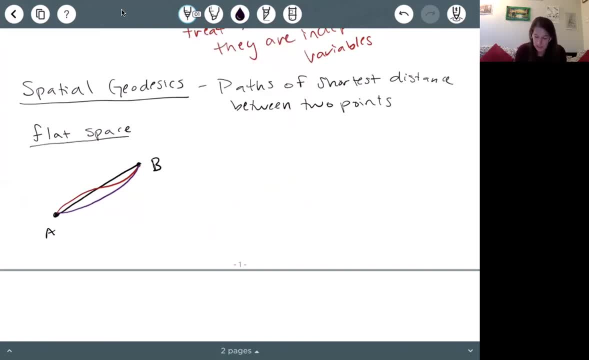 Now in flat space. this problem again, we've all seen it. But maybe we're in flat space and maybe there was some obstacle in the middle and then the path has to go around that obstacle. So then that would be a slightly less trivial problem. 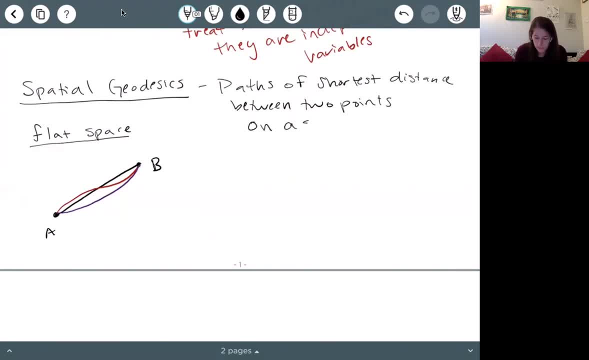 Or maybe we were on the surface of a sphere and we're trying to find the the shortest distance between point A and point B on the surface of a sphere, which now, this is a less obvious problem if you're constraining your path to be on the surface.